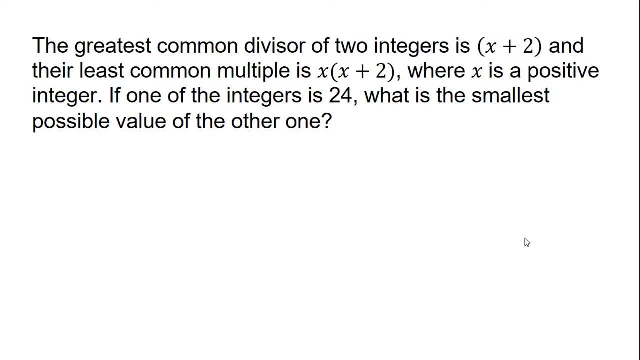 Hello everyone, welcome back. Today. in this video I'm going to be solving this example. So let me read the example first. The greatest common divisor of two integers is x plus 2, and their least common multiple is x times x plus 2, where x is a positive integer. If one of the integers 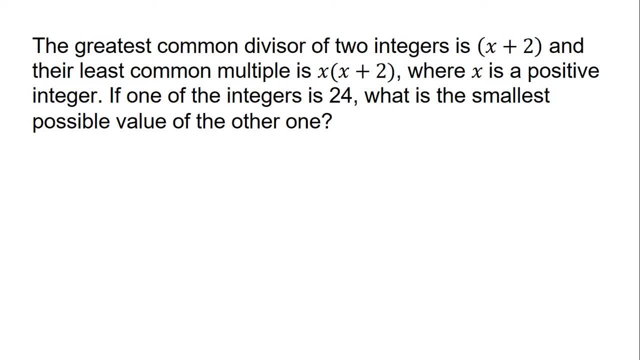 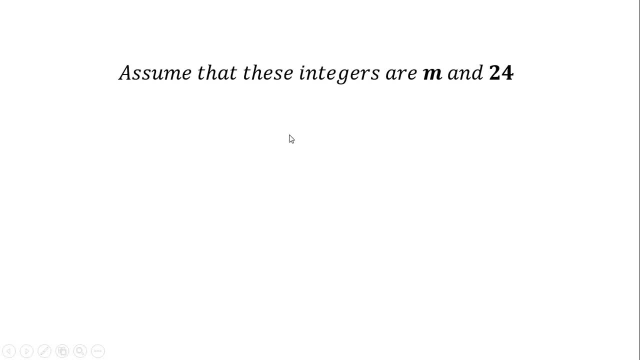 is 24, what is the smallest possible value of the other one? Okay, so, so it is given that these integers, one of these integers is 24, so let's say that the other one is M. So we know that M times 24 is equal to greatest common divisor of these two numbers times least. 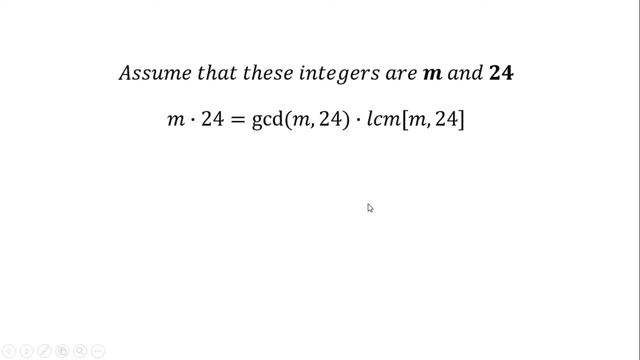 common multiple of these two numbers numbers. it is a very useful property in number theory. the product of two numbers is going to be equal to the product of their greatest common divisor and least common multiple. okay, so the greatest common divisor is given in the question and least common multiple is also given in the. 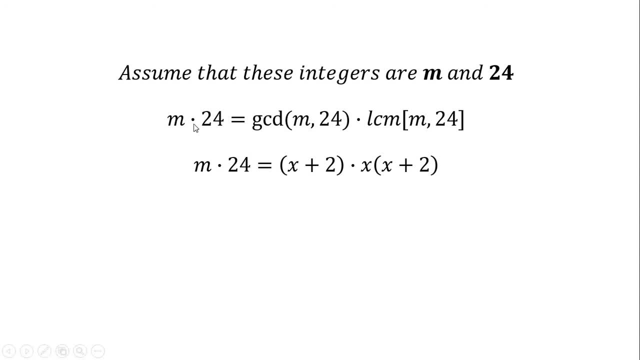 question. so now the expression is going to be: M times 24 is equal to X plus 2 times X times X plus 2. greatest common divisor is X plus 2 and least common multiple is X times X plus 2. so let's, let's. 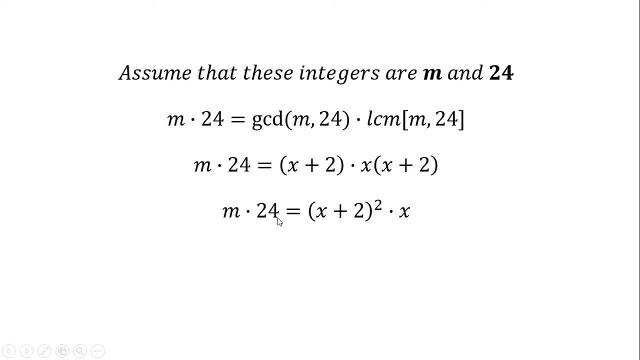 rewrite this expression, we are going to get M times 24 is equal to X plus 2 squared times X, because we have two X plus twos. as you see, X plus 2 times X plus 2 is X plus 2 squared and X, and we divide both sides by 24 to get M. so M is equal to X plus 2 squared times X, divided by 24. 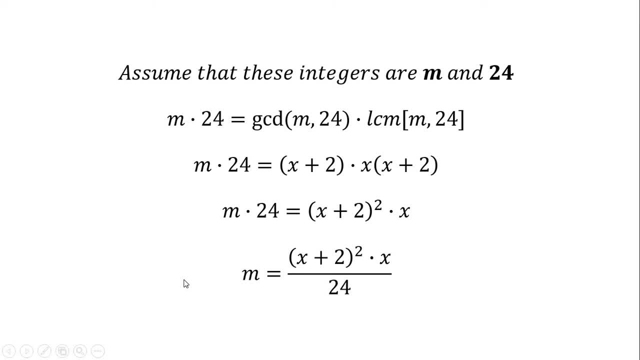 so we are going to try to find the smallest possible value of M. it is also given in the question that X is an integer. so in order to find the smallest possible value of M, we should find the smallest possible value of the denominator. but we should be careful because M must be also an integer. so in order to find the 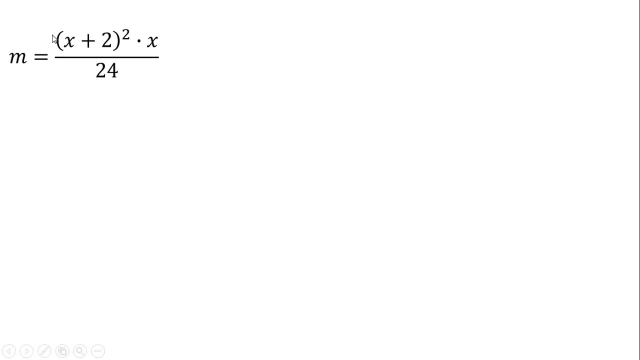 smallest possible value of the denominator. we can give X the value of 1, and then we can check M. if it is an integer, that's going to be our answer. if it is not an integer, then we can give X, 2 and then 3 and then 4 until we get the. 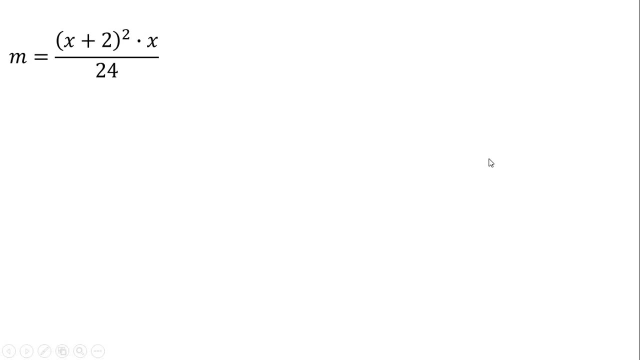 answer until we get M, an integer. alright, so let's say that X is equal to 1. so when X is equal to 1, so 1 plus 2 is 3.. 3 squared is 9, 9 times 1 is going to. 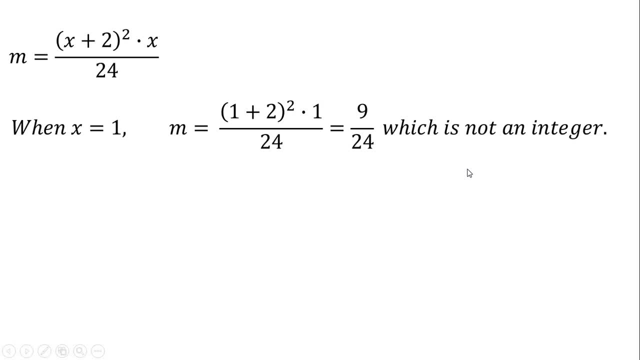 be 9.. 9 over 24 isn't an integer, so let's say that X is equal to 2. so in this case this is just an integer of a unit, but in Which paper is associated with X case M equals 2 plus 2 squared. 2 plus 2 is 4, 4 squared is 16, and 16 times 2 is 32, but 32 over 24. 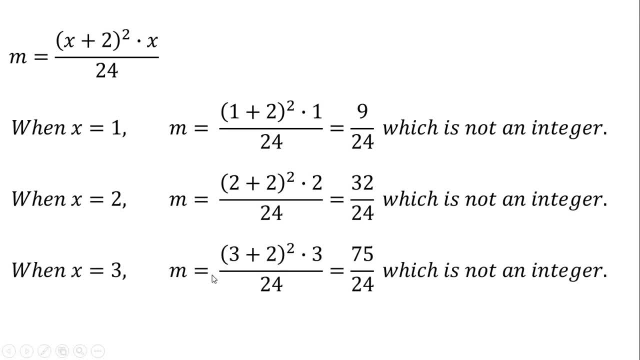 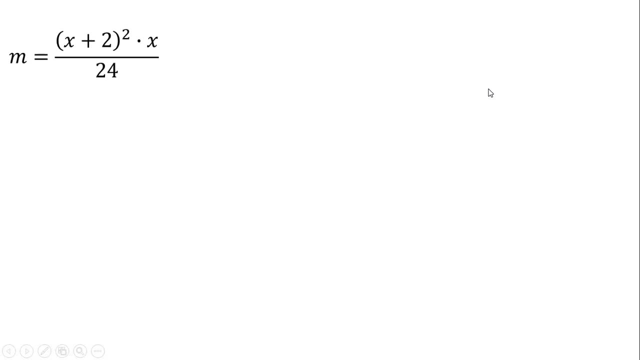 is not an integer when X is equal to 3. so M is going to be: 3 plus 2 is 5. 5 squared is 25, 25 times 3, 75. but 75 over 24 is not an integer. all right, let's try 4. so when X is equal to 4, 4 plus 2 is 6. 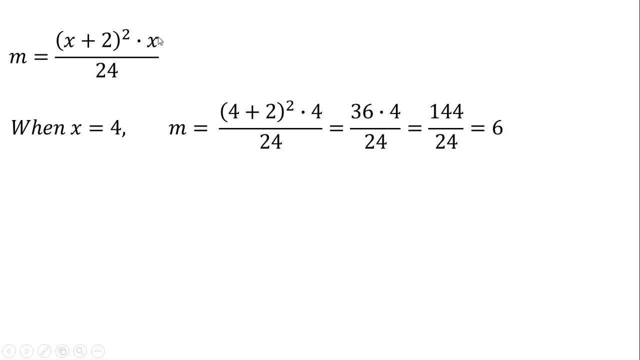 and 6 squared, is 36 times X, is equal to 4. so 36 times 4, which is 144, and 144 over 24 is equal to 6. so we get an integer that means M is 6. so let's get back to the question. all right, this is our question. if one of the integers 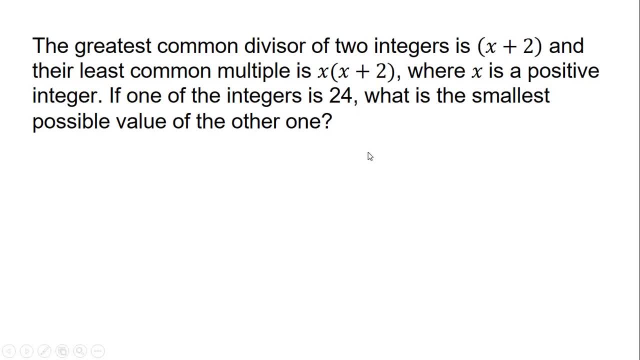 is 24. the smallest possible value of the other one is going to be 6, so 6 is the answer.